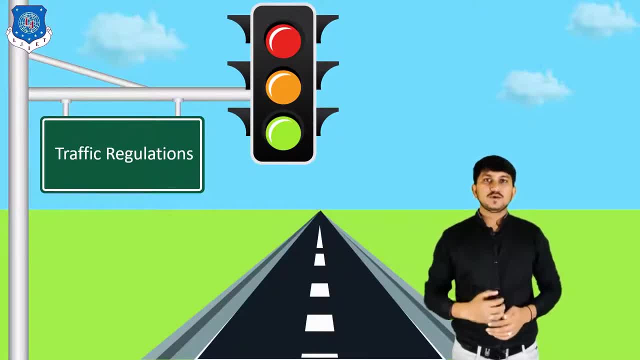 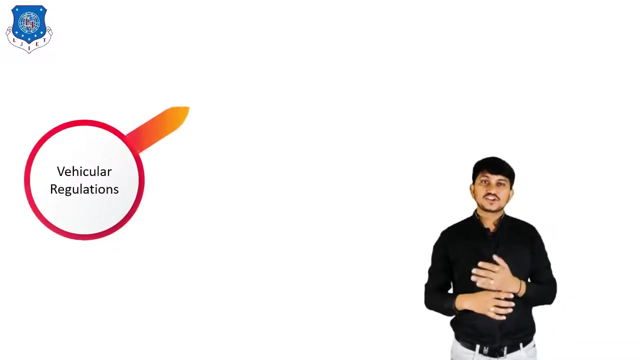 It is essential to impose adequate traffic regulations. So basically it is divided into three parts: First is Vehicle Regulation, Second is Driver Regulations And third is Road User Regulations. First let's see what are the Vehicle Regulations are. So to understand it, first we have to do registration of any vehicle. 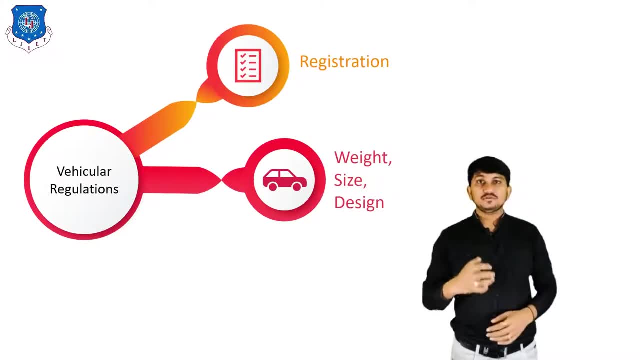 Which is known as RC Book. Then after we have to classify the vehicles according to their weight, size and design. Say, for example, if I talk about four-wheeler, Then it can be separated as heavy trucks. also, Even size and design of normal car and heavy truck is different. 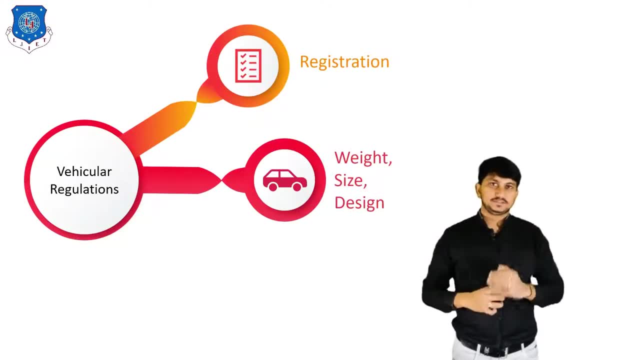 So we have to keep all the constraints in mind. Lastly, we have basic knowledge of construction of any vehicle. Even insurance of any vehicle plays a key role, While we want to claim it. So this is all about Vehicle Regulation. Now let's discuss our second part. 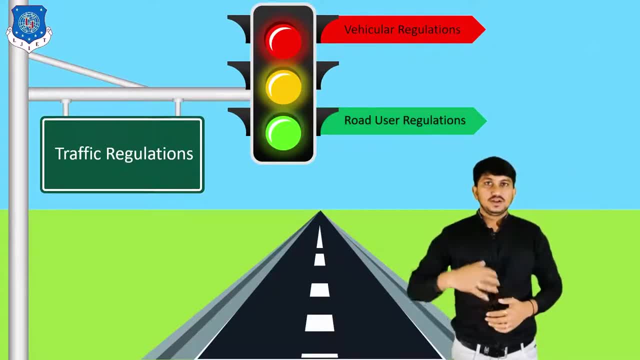 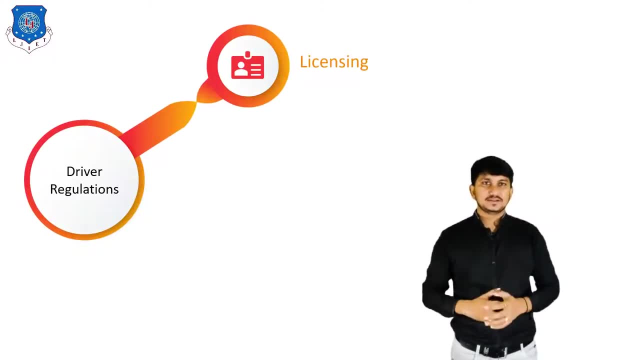 Which is Driver Regulations. So Driver Regulations can be done by licensing. As we know, a person must give driving test to get license, Where the driving skills are tested, And without license, driving any vehicle is a crime. Next is physical fitness and age of a driver that matters. 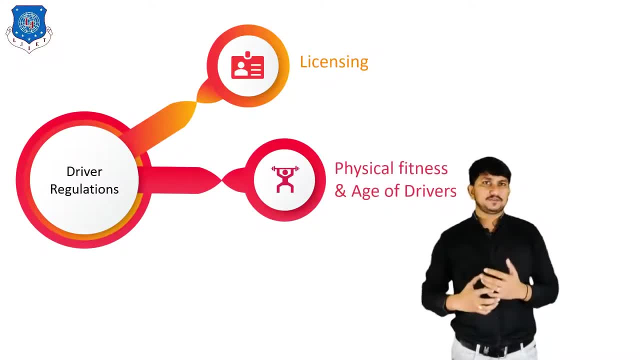 Say, for example, we prefer experienced driver Who is not too young and not too old. Because of this age, physical condition, as well as quick decision taking skill, reduces, While in younger stage with aggression, chances of accident are still there. And lastly, we will discuss about disqualification and endorsement of licenses. 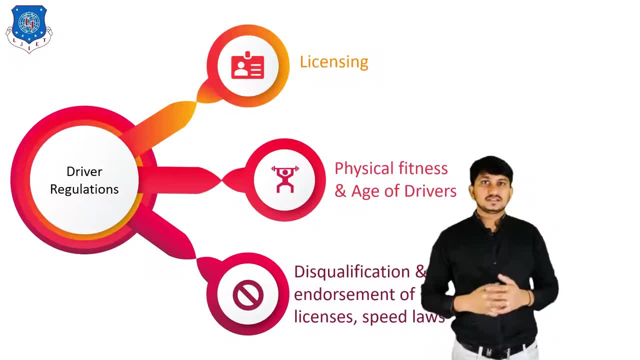 Of licenses and speed laws. Murdering offenses can incur fines and endorsements. An endorsement on your driving license means that you have been given points Which will remain on your license until they expire. Depending on the type of offense committed. This is usually 4 or 11 years. 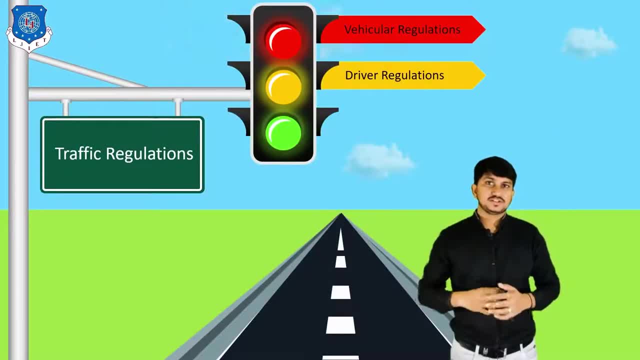 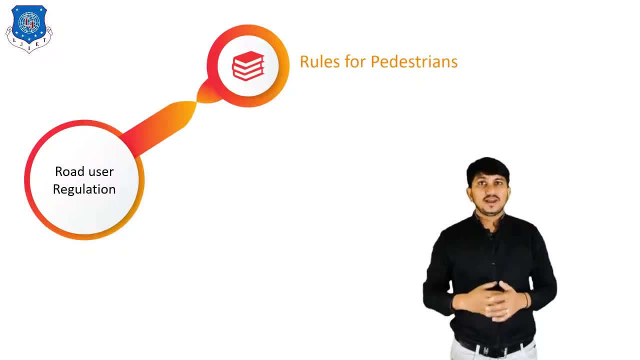 Now, next is Road User Regulations. Here we have to also think for pedestrians Crossroads. where there are pedestrian crossings, Always walk on the footpath. Where there is no footpath, walk in the right side of margin of the road. 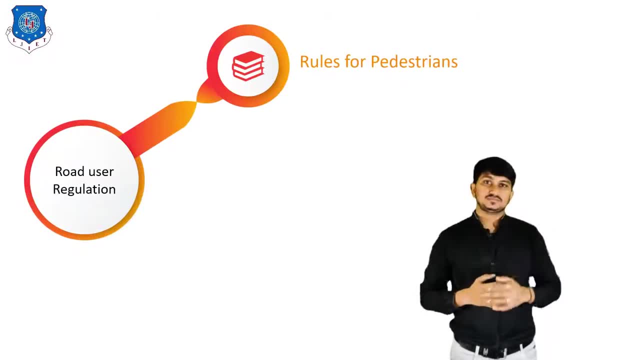 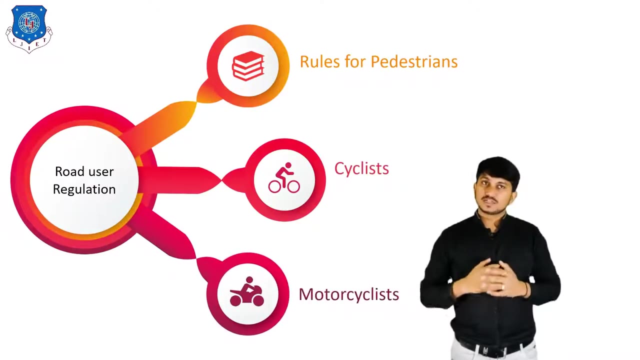 So that you can see the traffic coming in the opposite direction. Next is about cyclist. We should provide separate route for cyclist To ensure their safety and comfort on the road. Last but not the least, We should provide facilities to motorcyclist also. 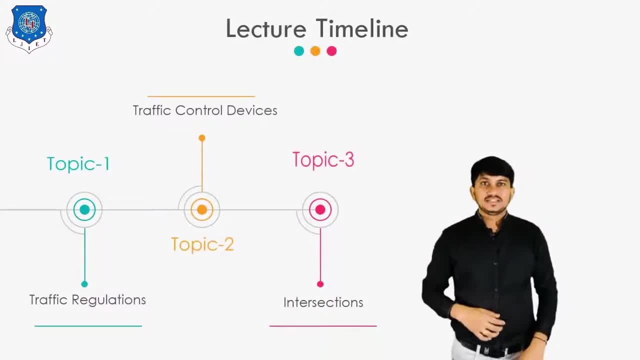 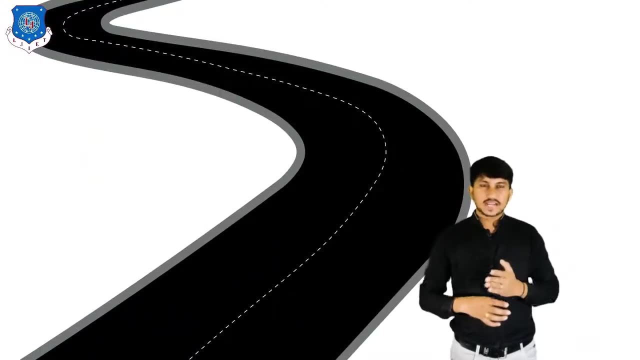 Now let's move to our second topic, Which is Traffic Control Devices. The various aids and devices which are used to control, regulate and guide traffic May be called as Traffic Control Devices. Broadly, these fall into 5 categories. First is Traffic Sign. 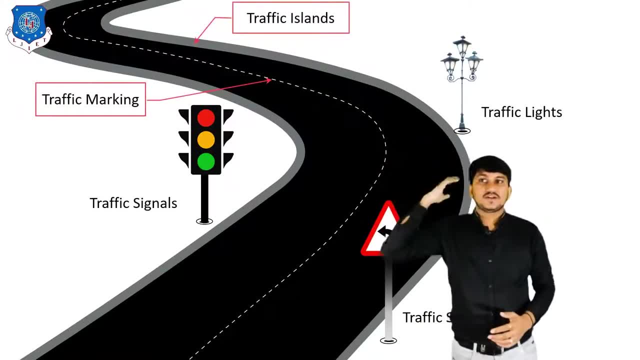 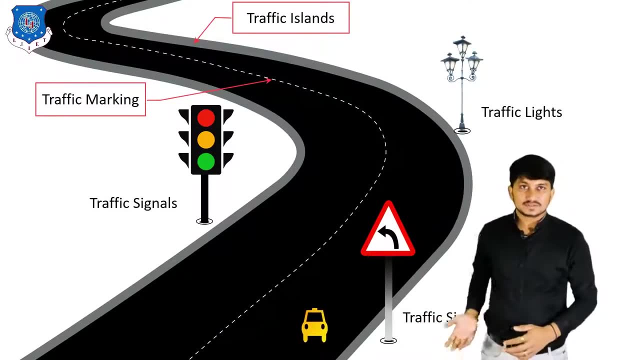 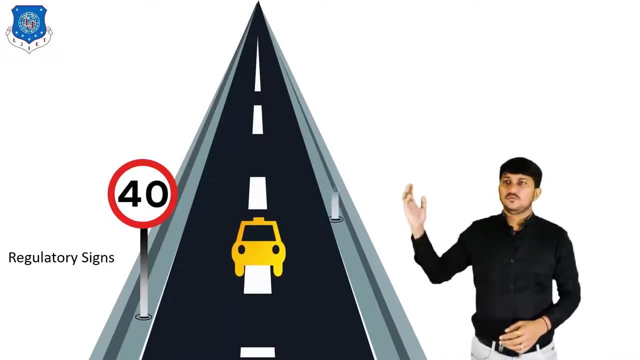 As you can see, Second, Traffic Signal, Third, Traffic Light, Fourth, Traffic Marking And fifth is Traffic Islands. Now let's discuss Traffic Sign first. So basically It is classified as Regulatory Sign, Warning Sign. 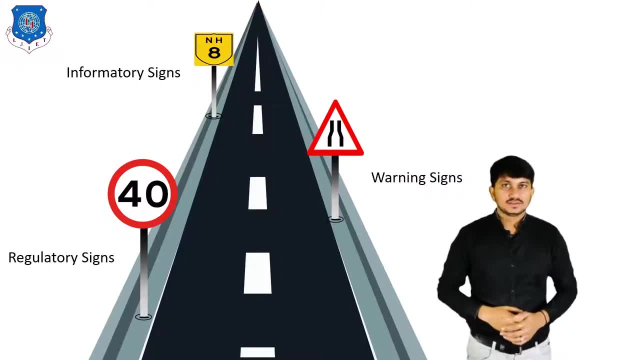 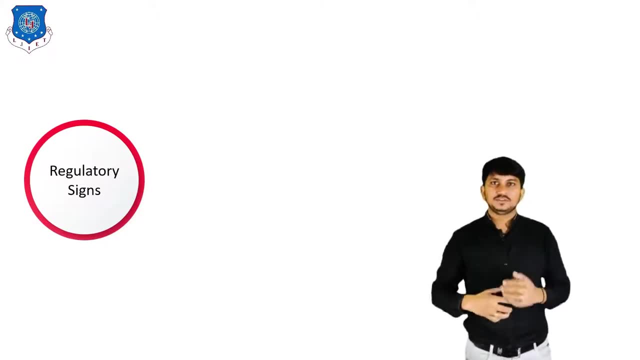 And Informatory Sign. So let's discuss Regulatory Sign first. Regulatory Signs are meant to inform the Road User of certain laws, regulations and prohibitions. It is further classified into Two types, Where First is Directional Road Sign. 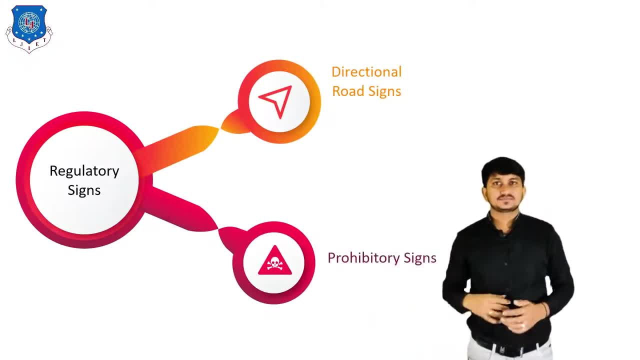 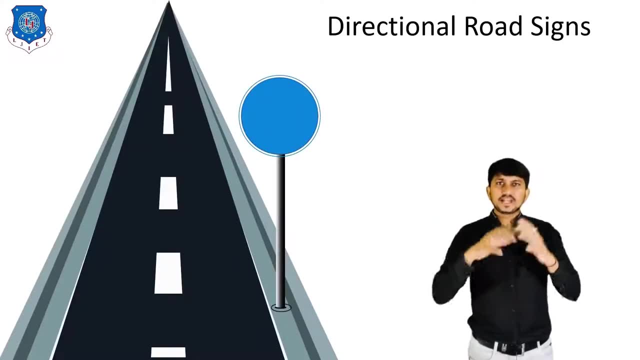 And Second is Prohibitory Road Sign. Here Directional Road Sign Have Blue Background And White Symbol. Different type of Regulatory Road Sign are Like Compulsory Turn Left, As you can see on figure. 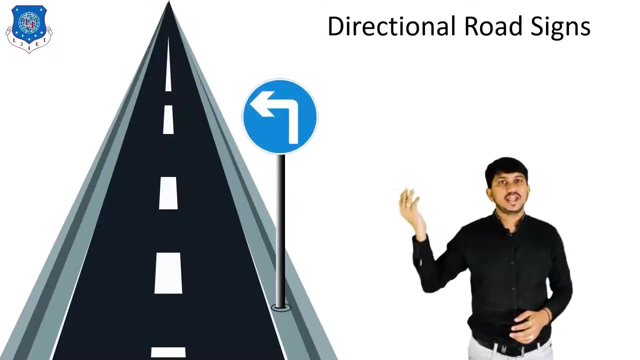 Compulsory: Turn Right. Compulsory Turn Left Ahead. Compulsory Turn Right Ahead. Compulsory- Keep Right, Keep Left. And Compulsory: Proceed Ahead. Now Let's discuss. 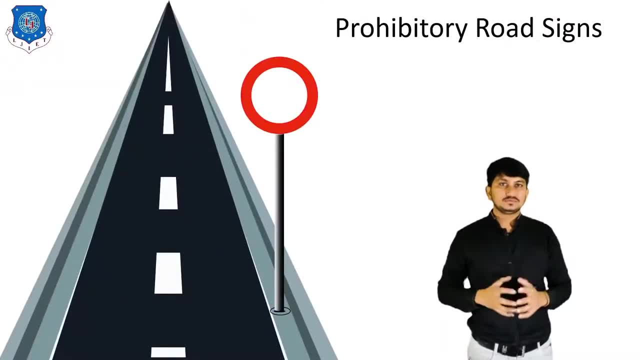 Prohibitory Signs. They have White Background, Red Border And Black Symbols. Different type of Prohibitory Signs are Like: No Parking, No Entry, No Left Turn, No Right Turn, No Overtaking, No Stopping. 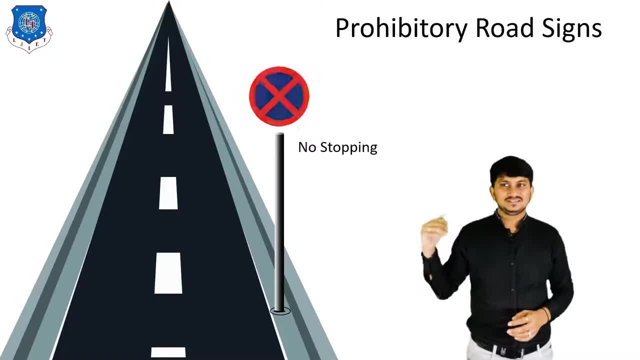 No U-Turn, No Horn, No Stopping, No Stopping, No Stopping, No U-Turn, No Horn, No Go, No Go, No Speed, No Go, No Speed, No Go, No Go, No Go. 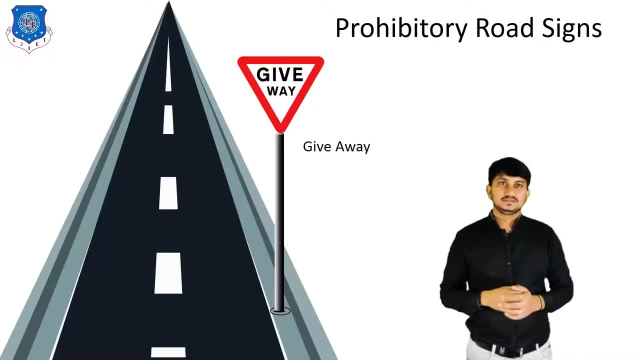 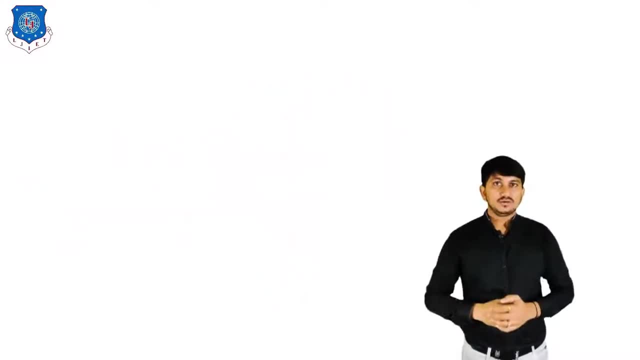 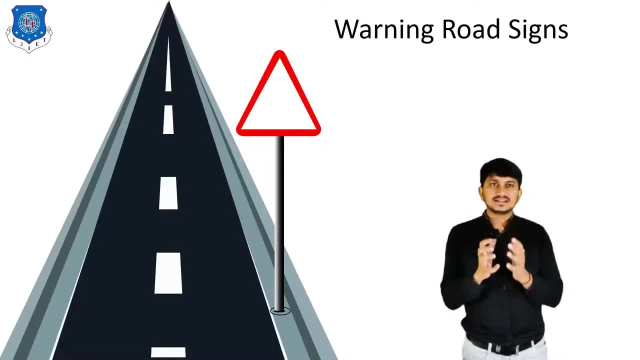 Which is Warning Sign. Warning Signs Are used to Warn that exist on or adjacent to the roadway. Warning signs are to great help in ensuring safety of the traffic. They have white background, red border and black symbols. Signs are to be located at sufficient distances, like 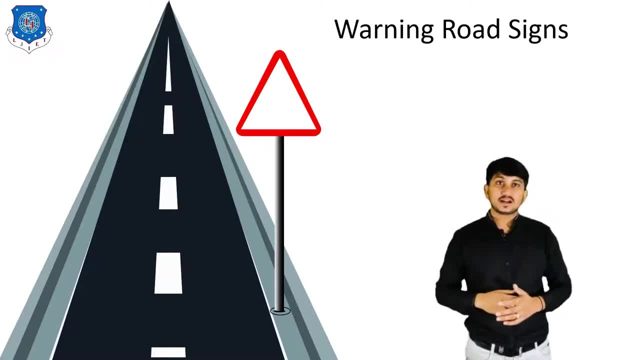 in National Highway or State Highway it will be around 120 m, in Major District Road is about 90 m. in Other District Road is at 60 m and in Village Road it is about 40 m respectively. Different types of warning signs are like. 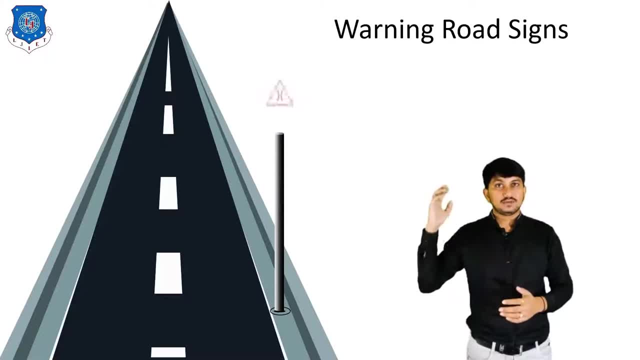 left hand curve, right hand curve, narrow bridge, man at work, uneven road, narrow road, roundabout in circle T-intersection, side road, right and cross road. Now, last type of traffic sign is Informatory Sign. Informatory Sign. 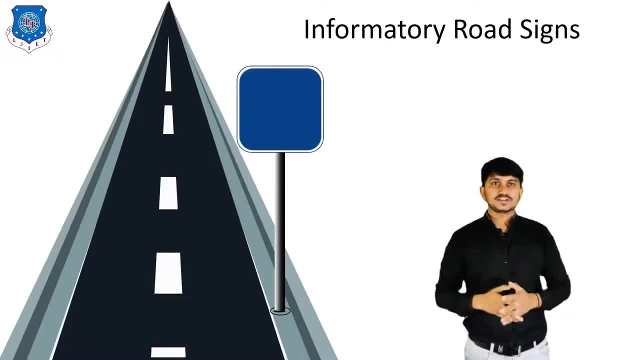 These signs are meant to provide information on direction, destination, roadside facilities, etc. to the road user. These road signs help a driver in saving time reaching destination without looking around. These signs are normally blue in colour. Different types of Informatory Signs are like: 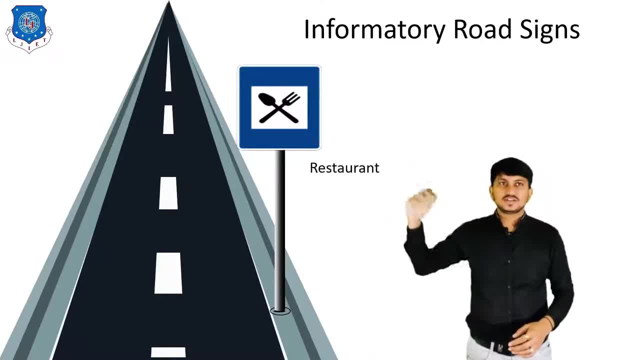 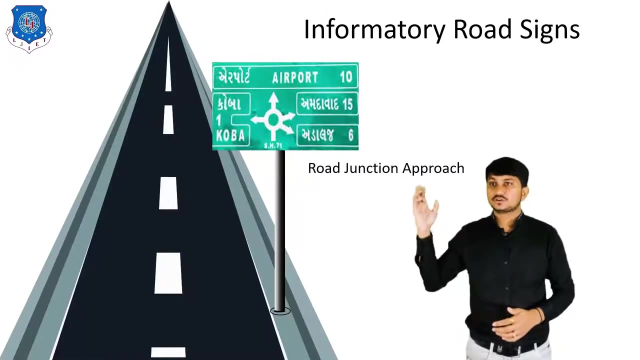 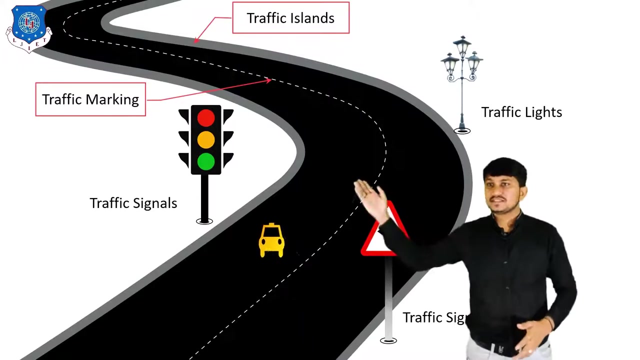 filling stations or petrol station, restaurants, hotels, parkings, first aid medical facilities, refreshments, hospitals, bus stop, route marker sign and road junction approach. These are the various Informatory Road Signs. Now let's discuss the next topic, which is Traffic Signal. 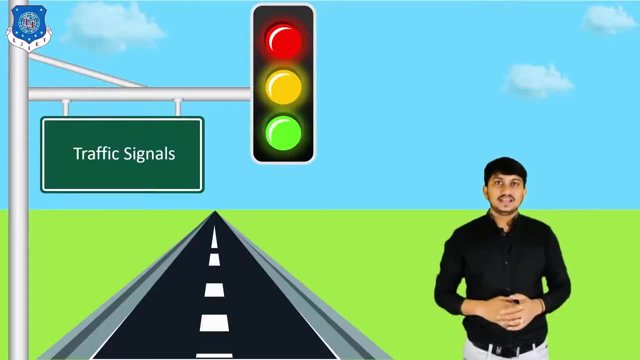 So a traffic signal is used as an instructing device that indicates the road user to act according to the displayed sign. The traffic signals ensure the road safety and, to make things simple to understand, These signals have been using a universal colour code. There are various types of traffic signals are used. 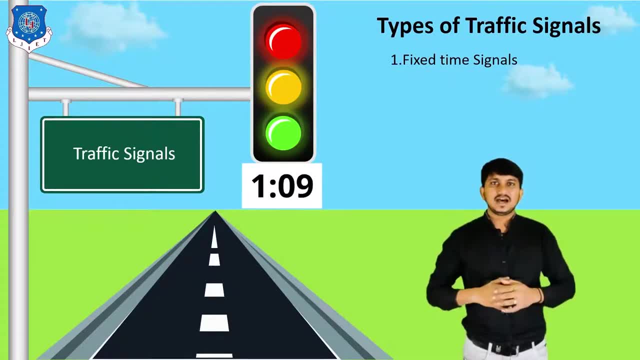 First is Fixed Time Signals. These signals are set to repeat regularly A cycle of red, amber-yellow and green light. Depending upon the traffic intensity. the timings of each phase of the cycle is predetermined. Fixed Time Signals are the simplest type of automatic traffic signals, which are electrically operated. 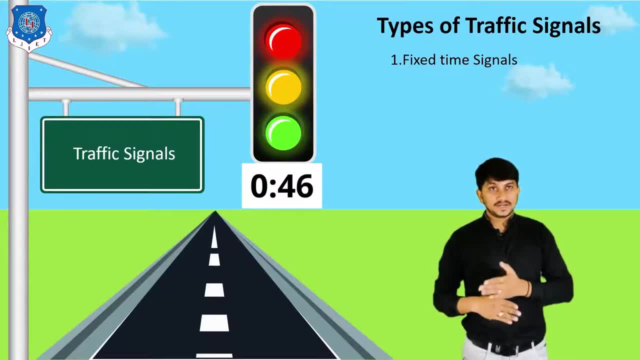 But the drawback of these signals is that the cycle of red, yellow and green goes on, irrespective whether on any road there is any traffic or not. Also, traffic in the heavy stream has to stop at the end phase. Second type is Manually Operated Signals. 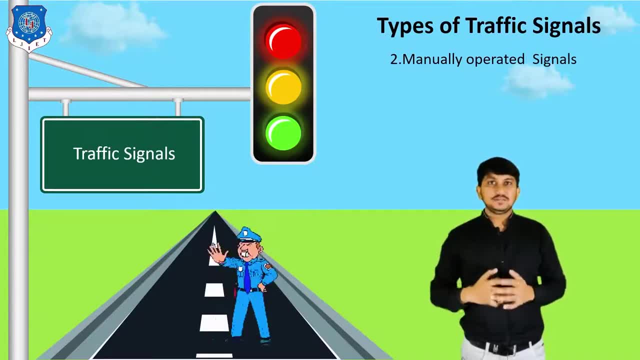 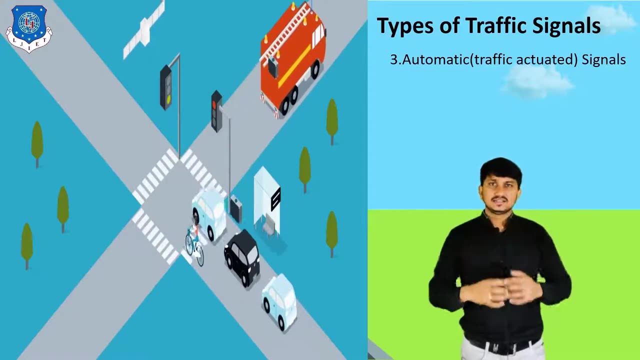 In these types of signals, the traffic police watches the traffic demand from a suitable point during the peak hours at the intersection and varies the timings of these phases and cycles accordingly. Third type is Traffic Actuated or Automatic type of signals. In these signals the timings of the phase and cycle are changed according to traffic demand. 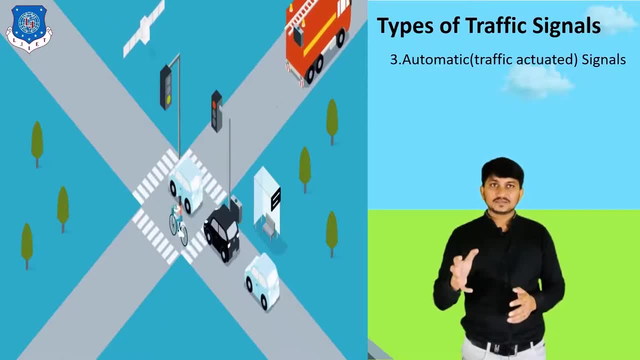 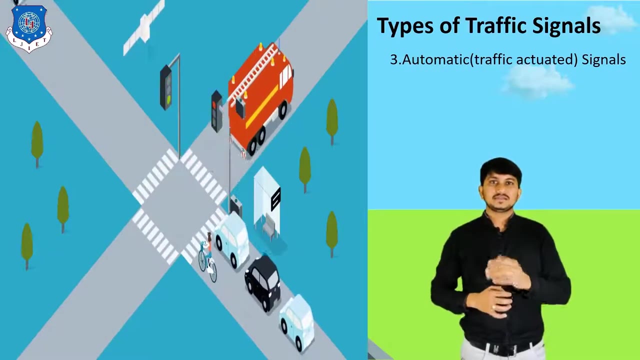 In semi-actuated signals, the normal green phase of traffic stream may be extended up to a certain period of time for allowing the vehicles to clear up the intersection. In fully actuated signals, computers assign the right of way for the traffic movement on turn basis of traffic flow demand. 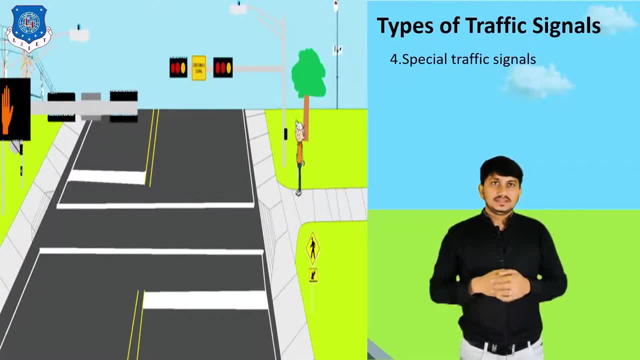 Fourth type is Special Traffic Signals. These signals are used to warn the traffic. When there is a red flashing signal, the drivers of the vehicle must stop before entering the nearest crosswalk, at the intersection or at a stop line, where marked Flashing of yellow signals are used to direct the drivers of the vehicle's traffic. 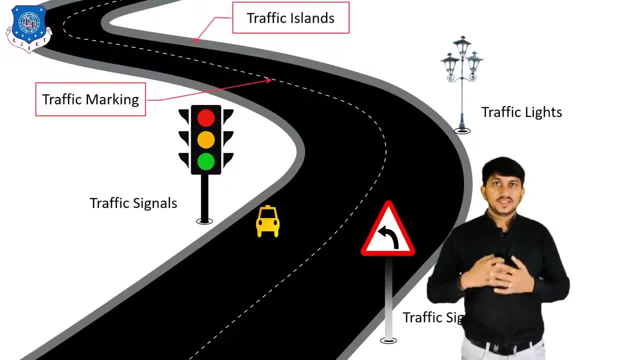 to proceed with caution. Now let's move to the next traffic control device, which is Traffic Light. It is a raised source of light on the edge of the road which is often mounted on a lamp column or a pole, either on the side of the road or within the median. 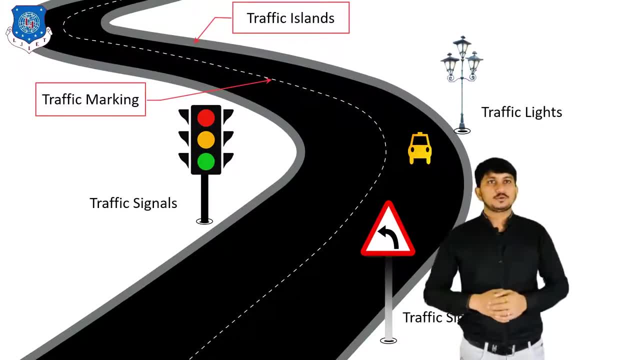 or suspended on a wire above the road to provide illumination. Street lighting can provide safety benefits to mid-block and intersection locations and can also improve safety for pedestrians, particularly at crossing points. Now let's move to the next traffic control device, which is Traffic Markings. 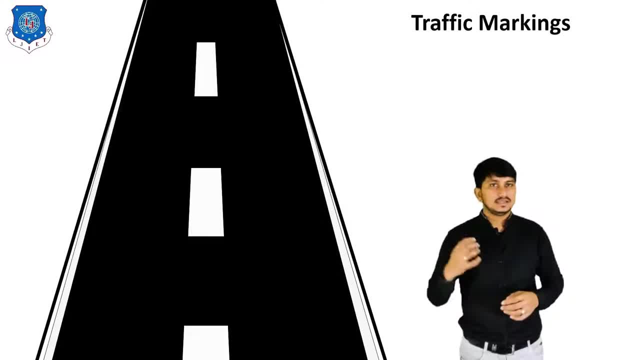 They are made of lines, patterns, words, symbols or reflectors on the pavement, curb, dividers or on the fixed objects. They are made using paints in contrast color and brightness. There are a number of types of roads: road markings. 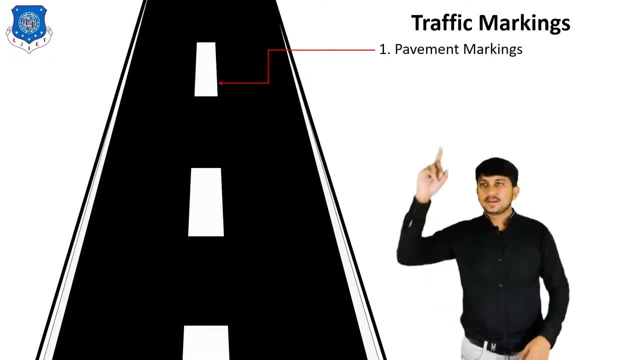 Let's discuss all in detail. First type is Pavement Marking. as you can see in the figure, White strips in the middle of the road pavement is known as pavement marking. These strips can be marked differently for different purposes. like here: it is marked as a dotted line. 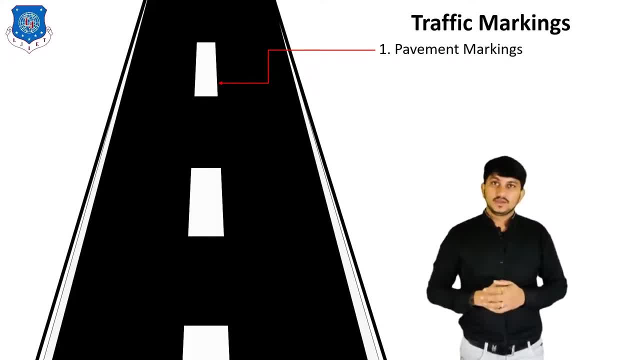 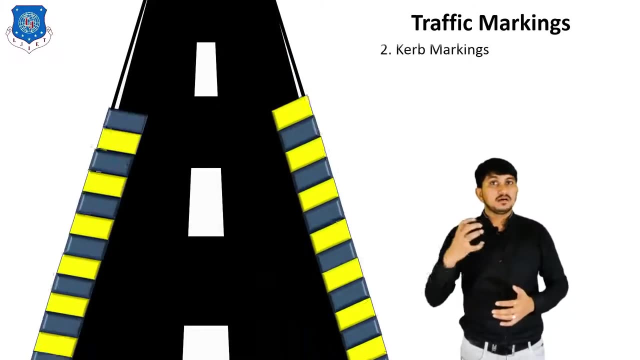 which indicates one can change the lane while driving, While solid line indicates one cannot change the lane or overtaking the vehicles. It helps in smooth and harmonious flow of traffic along guided lanes. Next type is Curb Marking. Here you can see black and yellow color strip. 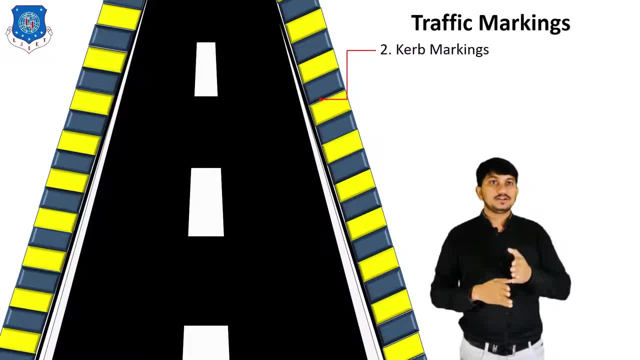 which is raised portion at the edge of the pavement along the side of the road which is known as curbs. These are the curbs. They are painted with either alternative black and white strips or in black and yellow strips. They divide pedestrian's walkway and roadway. 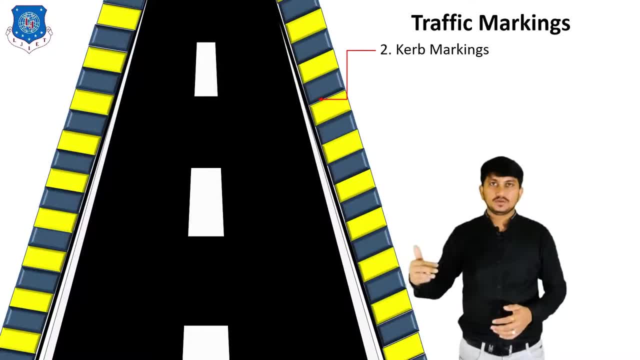 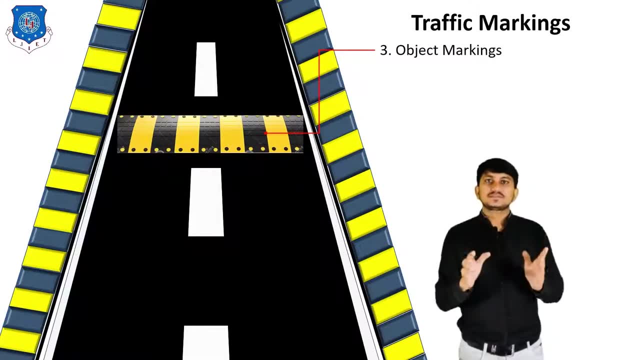 It helps to guide rainwater on the roadway to the drainage line. Now the next type is Object Marking. Sometimes, objects adjacent to the carriageway or roadway may pose some obstruction to the flow of traffic. Objects such as subway piers and abatements. 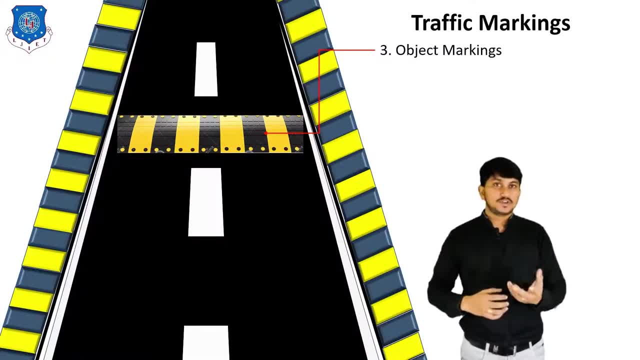 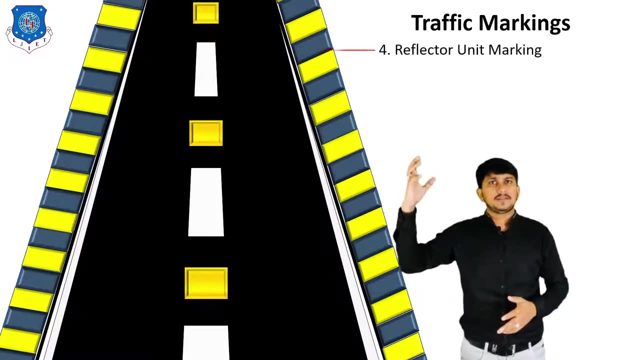 culvert, headwalls, small temple or a tree, These are the objects which are the obstruction. This causes serious hazards to the flow of traffic and must be marked to reduce the accident rate. Now, next type is Reflector Unit Marking. It is safety device used on roads which reflects with light at night. 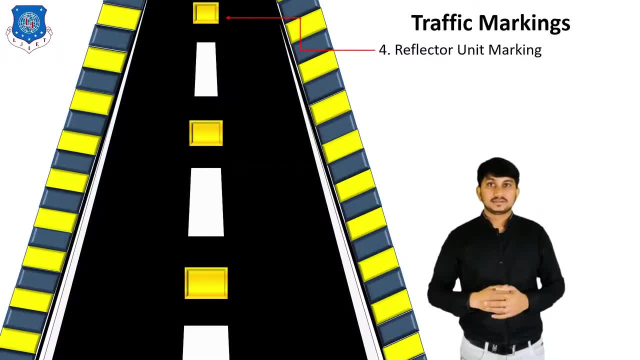 They are made with plastic, ceramic, thermoplastic, paint, etc. It is available in different shapes and colors. Mainly placed on the changing line of the lanes and edge of the pavement, It helps to identify boundary of lanes while night driving. Now, next type is Road Delineators. 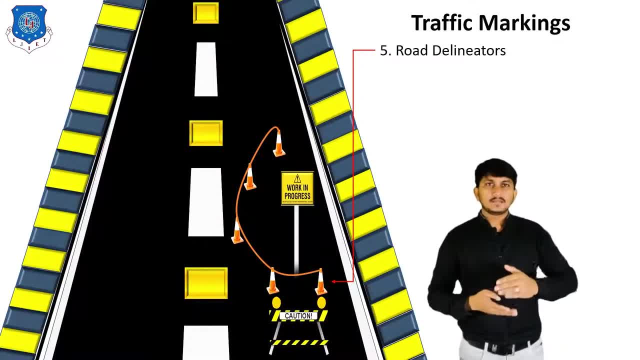 As shown in screen delineators are tall pylons similar to traffic cones, mounted on the road surface or along the edge of the road. They are used to channelize the traffic. They are usually seen on dividers of the bridges and for maintenance work. 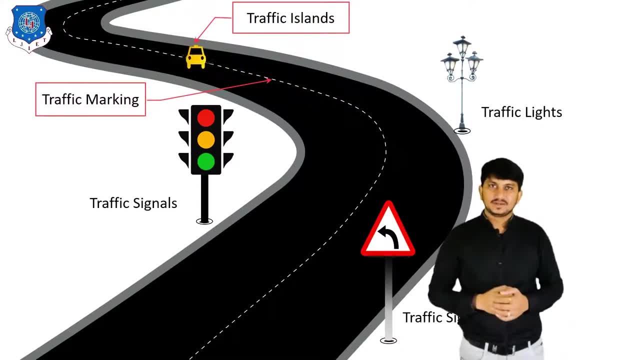 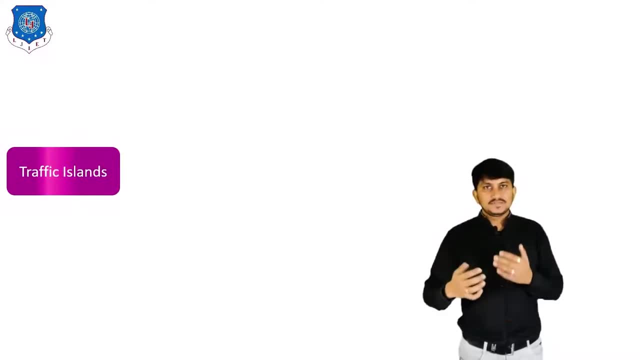 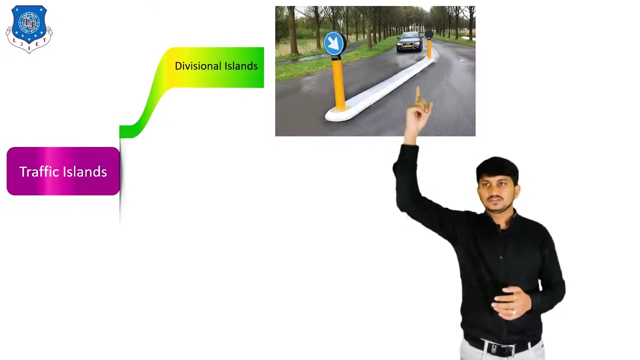 Now let's discuss Traffic Islands. Traffic Islands are raised area constructed within the roadway to establish physical channels through which the vehicular traffic may be guided. This can be classified into four types based on functions. First type is Divisional Islands. As you can see, this is a divisional island, is also called as divider. 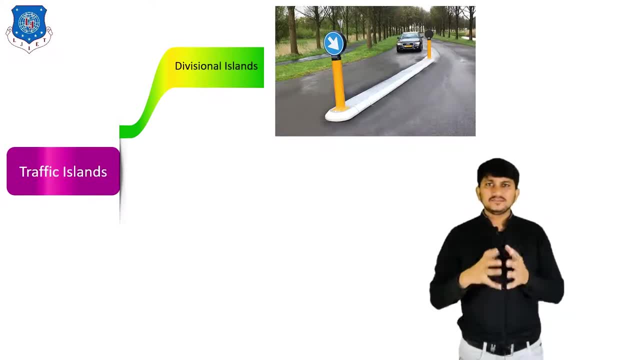 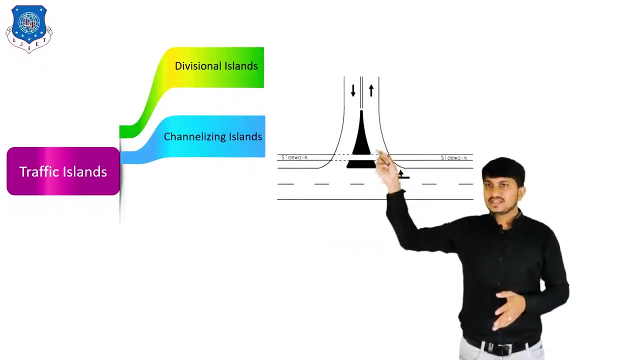 They are intended to separate opposing flow of traffic on a highway with four or more lanes By thus dividing the highway into one-way road, so that the head-on collision can be eliminated. Next is Channelizing Islands. These are the channelizing islands. They are used to guide the traffic into proper channel. 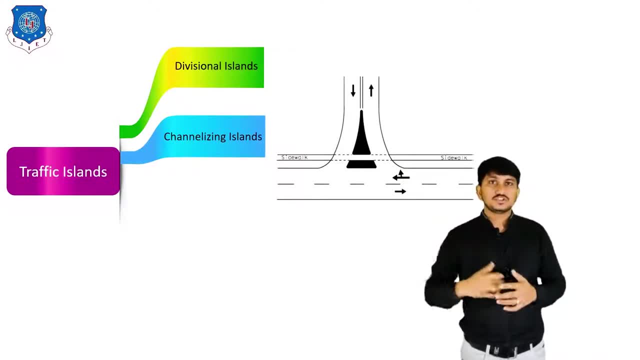 through intersection area. It is the separation or regulation of conflicting traffic movements into definite path of travel by traffic islands or pavements marking to facilitate the safe and orderly movements of both vehicles and pedestrians. Next is Pedestrian Islands. These are the pedestrian islands. 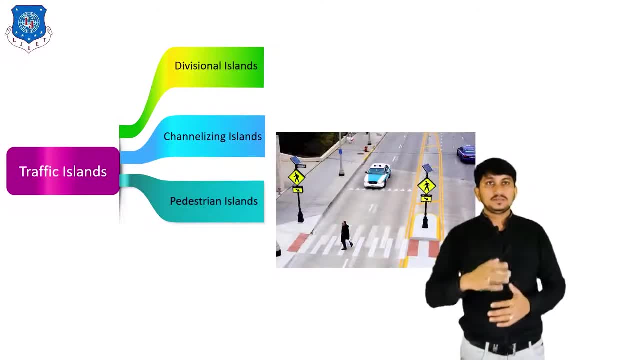 It is a small section of pavement or sidewalk completely surrounded by asphalt or other road material like concrete, where pedestrians can stop before finishing the crossing road. It is typically used when a street is very wide, As the pedestrian crosses can be too long for some individuals to cross in. 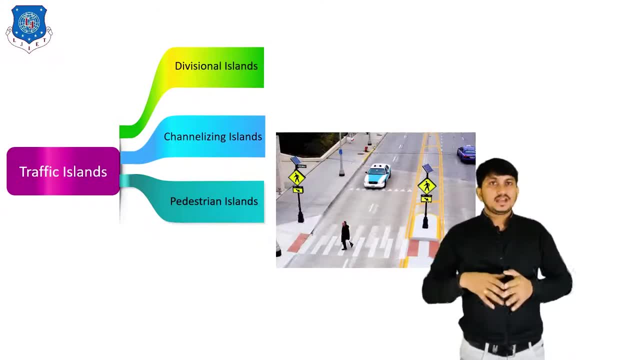 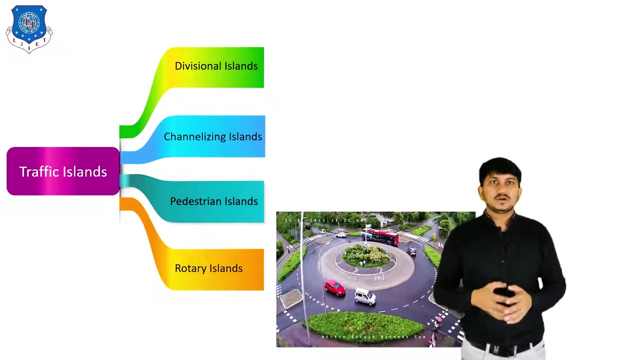 They may also be seen on the roads with high speed limits. It reduces the exposure time experienced by pedestrians in the intersection. Last is Rotary Islands. The raised platform of suitable shapes built on the road intersection are called as Rotary Islands. This is the Rotary Island. 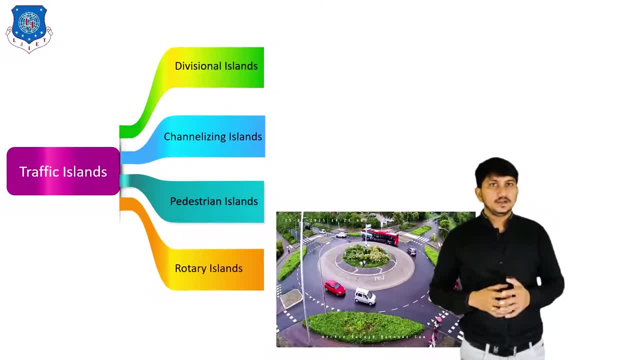 The main objects of providing a rotary are to eliminate the necessity of topping, even for crossing streams of vehicles, and to reduce the area of conflict. The crossing of vehicles is avoided by allowing all vehicles to merge into the stream around the rotary and then to diverge out the desired radiating road. 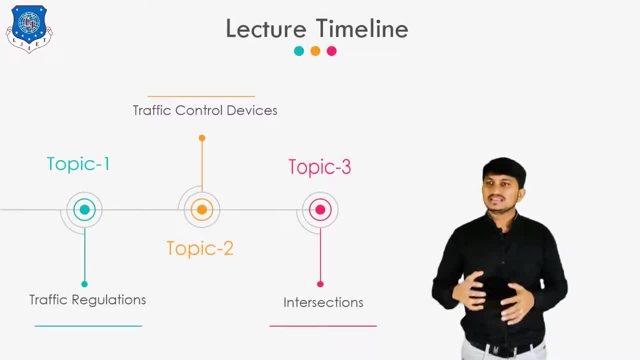 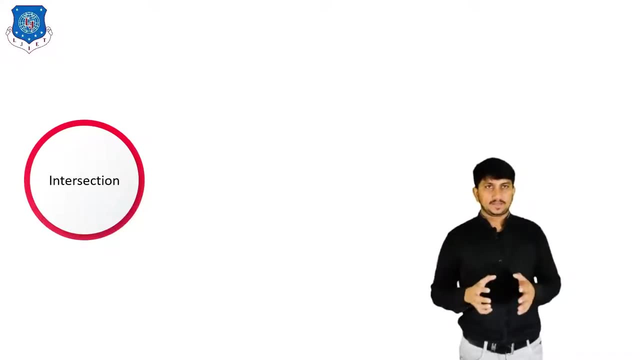 Now let's discuss the last topic of today's lecture, which is Intersection. So an intersection is defined as the general area where two or more highways join or cross Within, which are included the roadway, roadside facilities for traffic movement in that area, The efficiency, safety, speed, cost of operation. 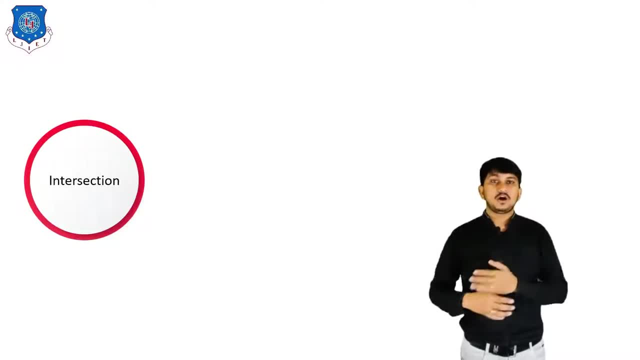 and capacity of road system very much depended on this intersection design. Various forms of intersections are like T-intersection, Y-intersection, multiple intersection, cross intersection and in skew intersection one inclined road is connected with the main road. Here skewed cross intersection is the combination. 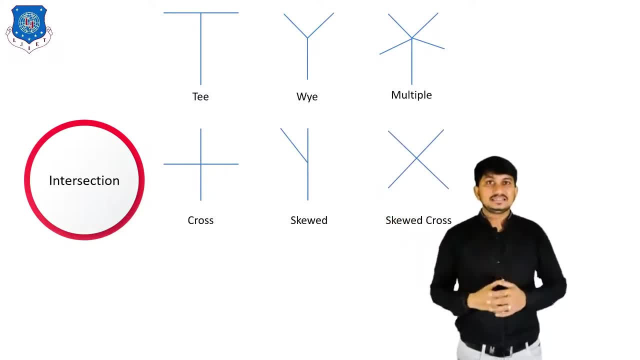 of cross and skewed. Staggered is different than cross intersection, as in cross road connected to the one point, while in staggered it is not connected at one point. It is in staggered or uneven manner. Last is Q-staggered intersection, which is the combination of staggered and skewed. 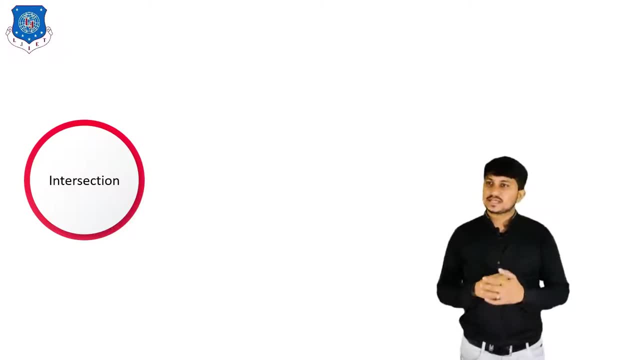 Now let's move to the classification of intersections. It is classified into two broad groups. First is intersection at grid and second is grid separated intersection. First we will discuss intersection at grid. In this all roads meet at the same level. This intersection can be further classified into three types. 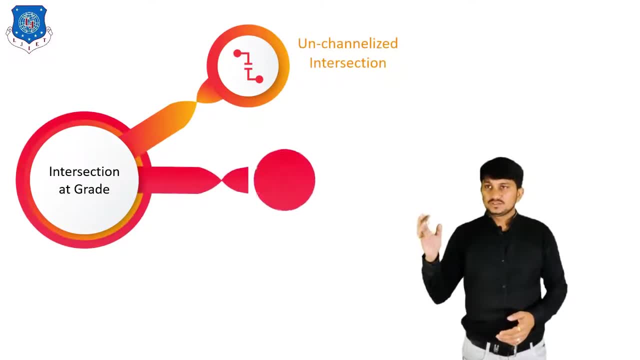 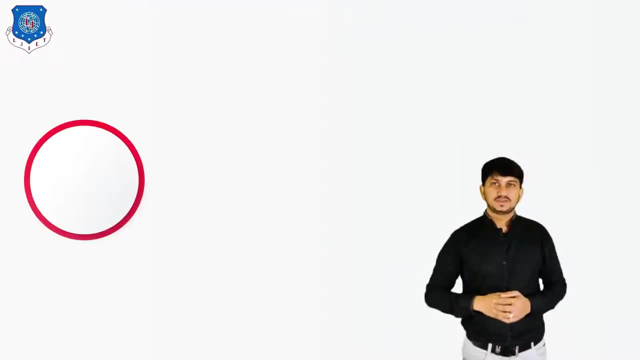 like un-channelized intersection, channelized intersection and rotary intersection. First is un-channelized intersection. In this type of intersection there is no provision of traffic islands or dividers to channelize the traffic flow. Let's see the examples of un-channelized intersections. 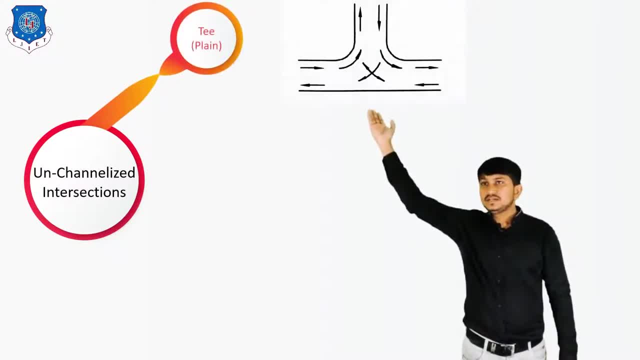 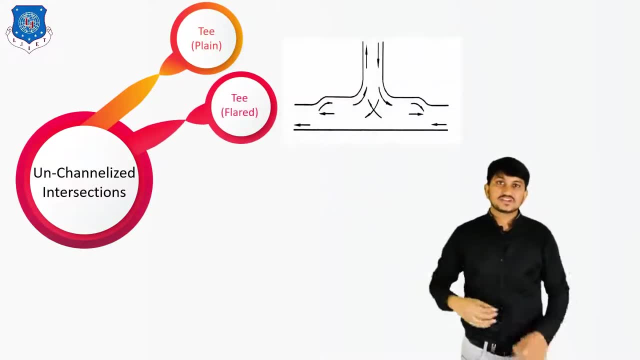 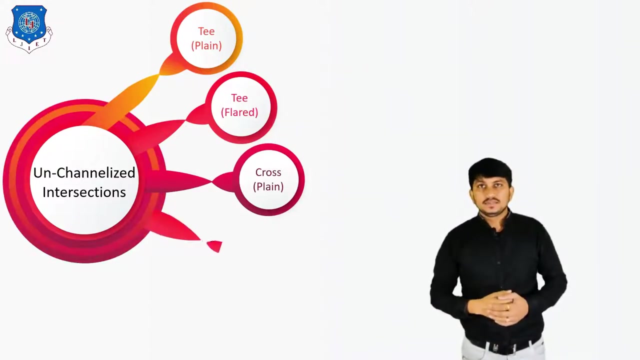 First is T-plane intersection, where there are no dividers in that. Second is T-flared intersection. Here in flared, at the intersection, the intersection width of the road is increased for less congestion of traffic. And the third is cross-plane intersection. Fourth type is cross-flared intersection. 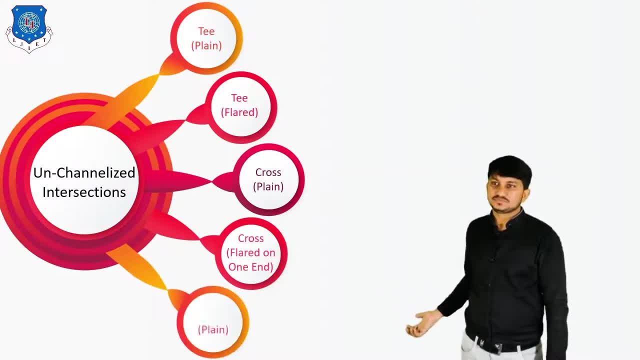 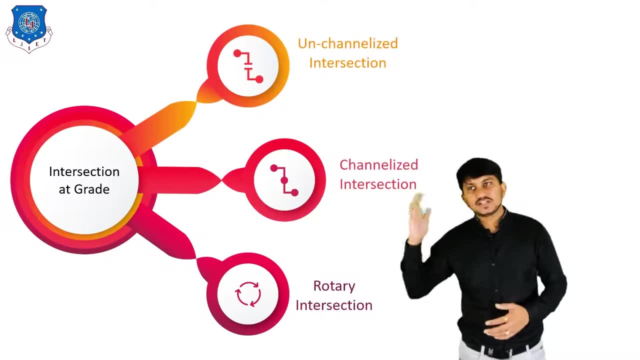 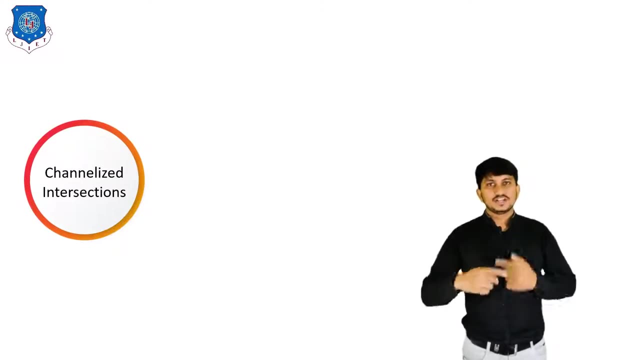 And the last is skewed-plane intersection. Now let's move to the second type of intersection at grid, which is channelized intersection. In this type of intersection, traffic islands or dividers are provided to channelize the traffic flow or regulate the traffic flow. Let's see some examples of channelized intersection. 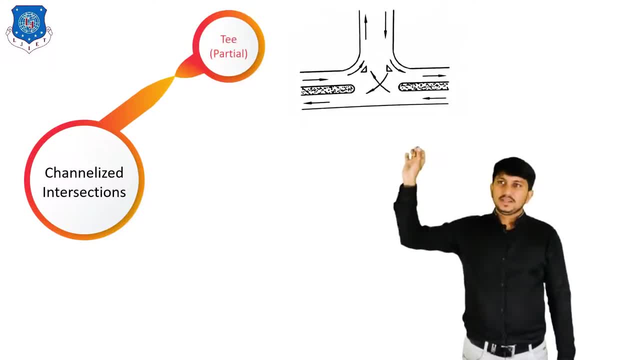 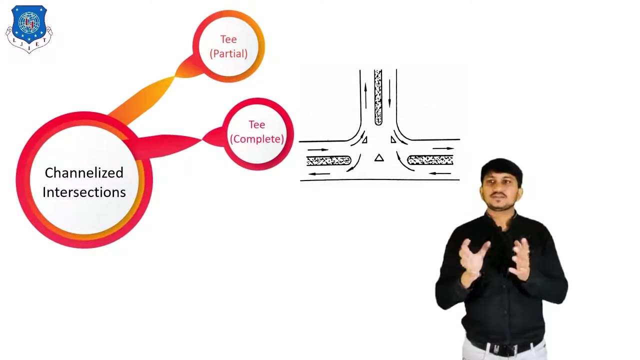 First is T-partial channelization. In partial channelization, the number of dividers is provided only on main roads, not on the minor roads. Now, the second type is T-complete channelization: intersection, in which all connecting roads have islands or dividers For proper traffic flow. 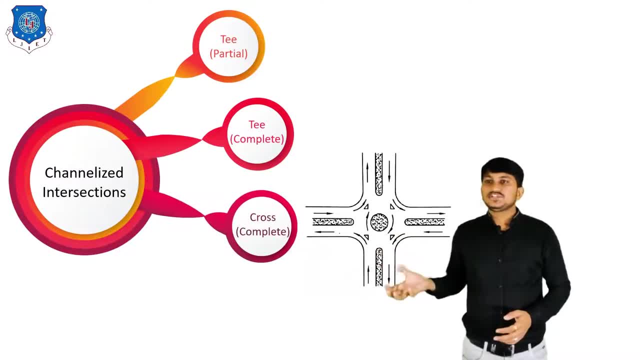 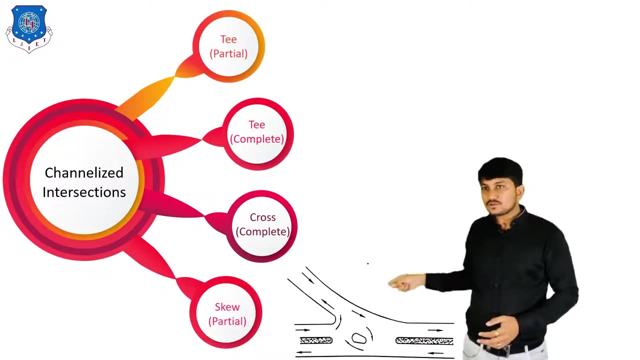 And next is cross-complete channelization. Here you can see in all roads number of dividers or islands are provided. And the last is skewed-partial channelization Because of partial- the inclined road or minor connecting road haven't have the dividers or islands. 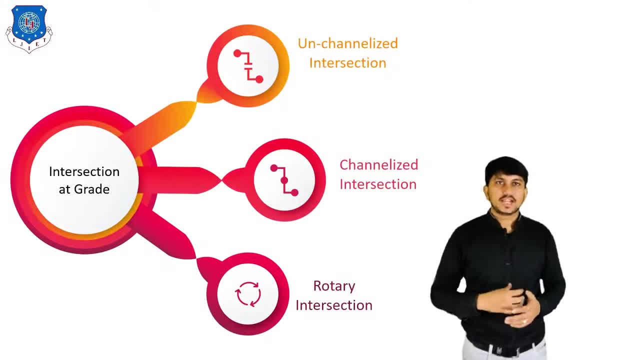 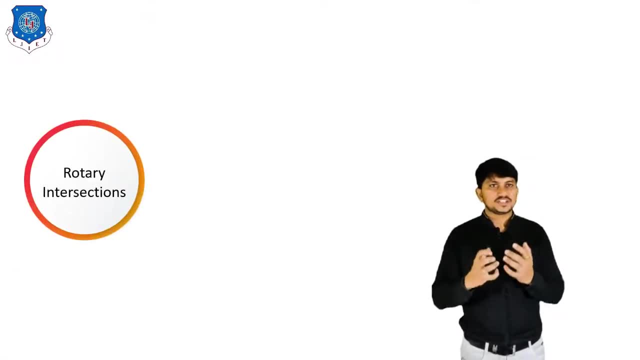 Now let's move to the third type of intersection, Third type of intersection at grid, which is rotary intersection. A rotary intersection is a specialized form of intersection at grid in which traffic moves in one direction around a central island, For keep to the left rule. 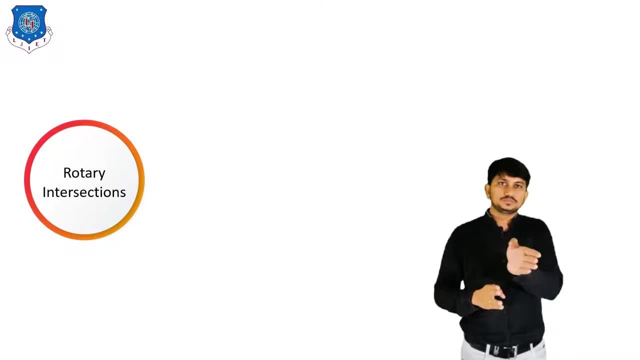 vehicles approaching in the intersection are forced to move round around the central island in an ordinary manner and wave out to the rotary into their respective desired direction. Let's discuss various types of rotary intersection. First is circular rotary intersection. Second is elliptical intersection. 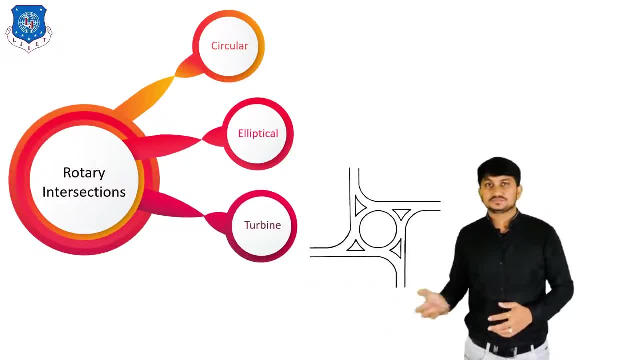 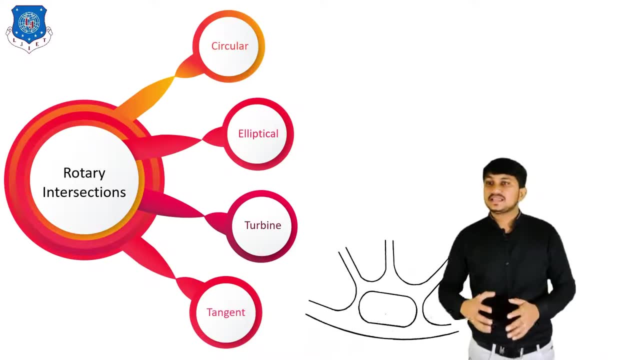 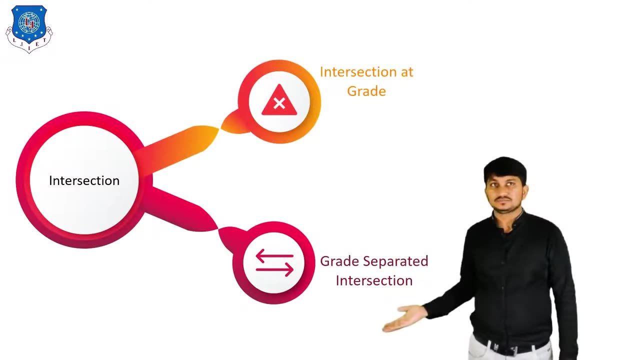 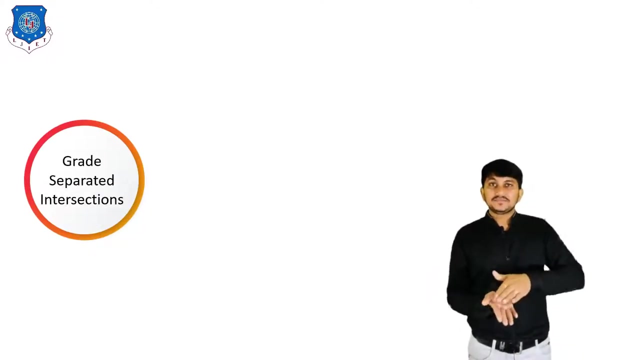 Third is turbine type of intersection And the last is tangent intersection. These all four types are based on their shapes. Now let's move to the second type of intersection, which is grade separated intersection. In this type of intersection, intersecting roads are separated by difference in level. 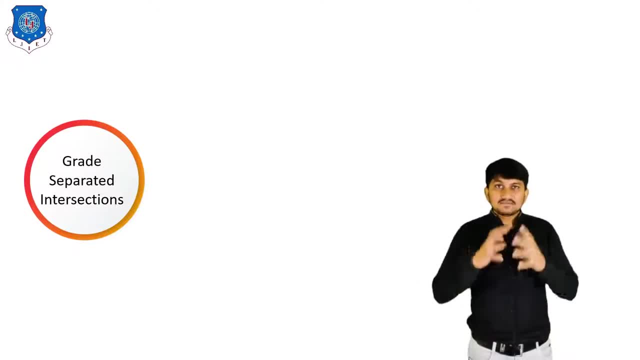 thus eliminating the crossing problem. This type of intersection cause least delay and hazard to the crossing traffic. It increases traffic safety and gives efficient operation of traffic flow. Let's discuss the example of grade separated intersection. First is diamond interchange, Which is a popular form. 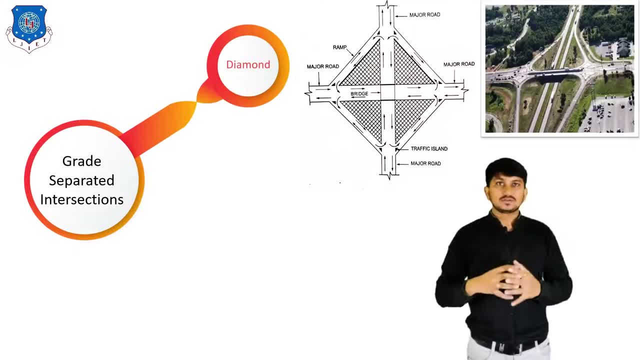 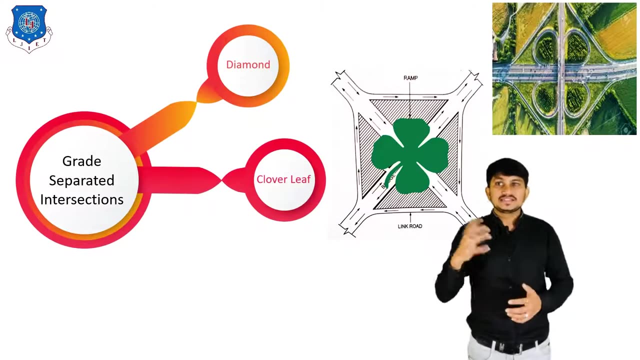 in urban location where major and minor roads are crossing at different levels. It is designed for a relatively narrow right of way of major road. Second type is clover leaf interchange. Its name comes from one leaf having same shape as you can see in figure. 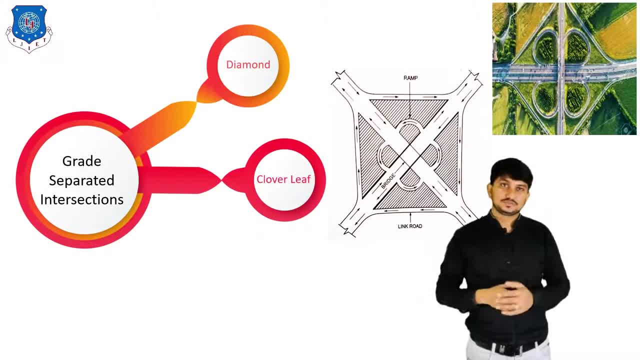 This is a four leg interchange with a single structure. It is a popular and used when two high volume and high speed roads are intersecting with each other. Its main advantage is that there are two points of entry and exit on each roadway. The first exit is provided. 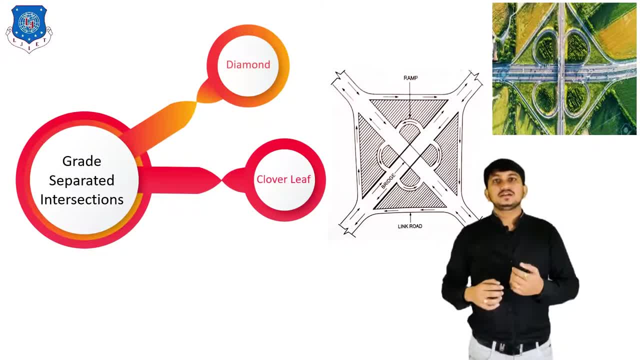 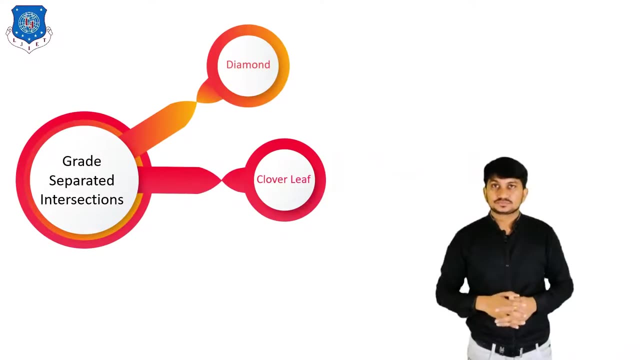 before the cross road structure allows right turn movements and the second exit, immediately after cross road structure, allows for the left turn movements. Its main disadvantage is that U turns are long and operationally difficult and slow. And the last is rotary island. It is the type of 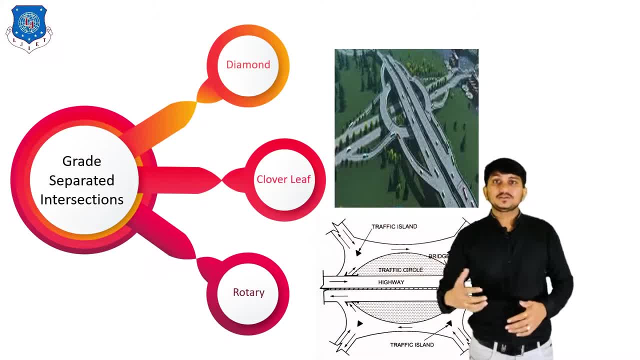 grade separated intersection. It is similar to the rotary interchange which is discussed just before this topic, Except in this type intersecting roads are not at the same level. It is also a four leg interchange which is used where land area is less and U turns are easy.